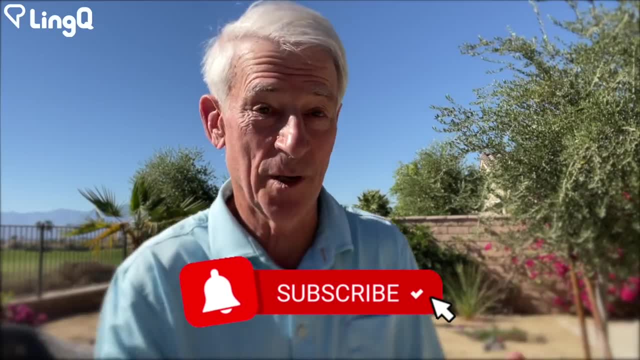 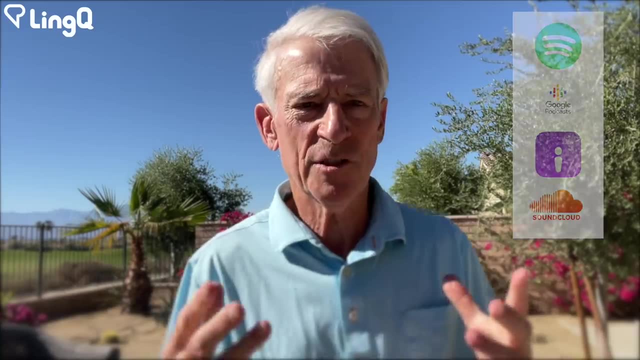 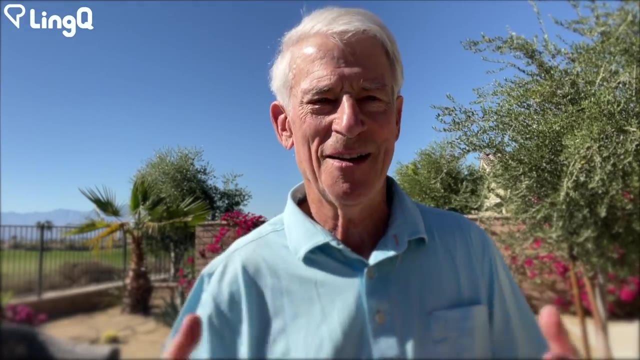 please subscribe And click on the bell for notifications And if you follow me on podcast service, please leave a review. So, first of all, why am I talking about problems? Because my whole filming setup is giving me nothing but problems. Last video I had 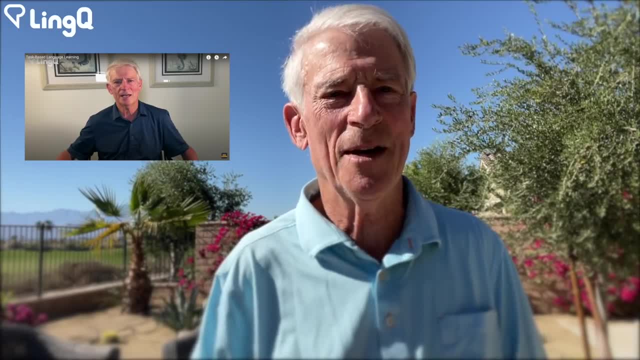 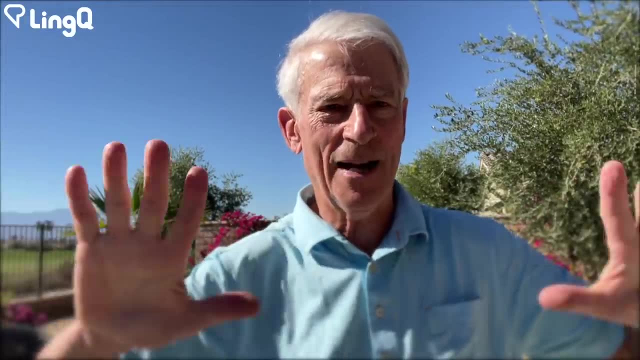 this reflection on those prints that I have in behind me. the time before that I filmed in front of the curtain, which didn't look very nice. I've ordered some hanging sort of backdrops, but haven't figured out how to pin them up yet, and then it will, at least. 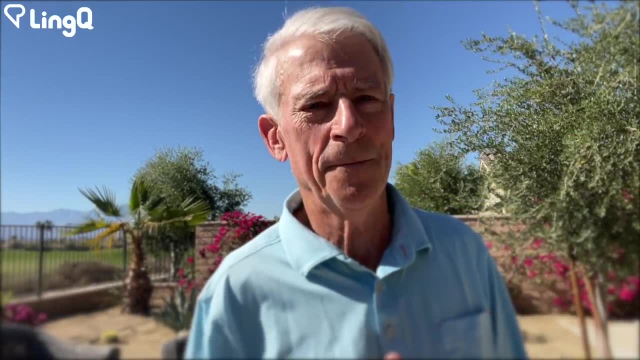 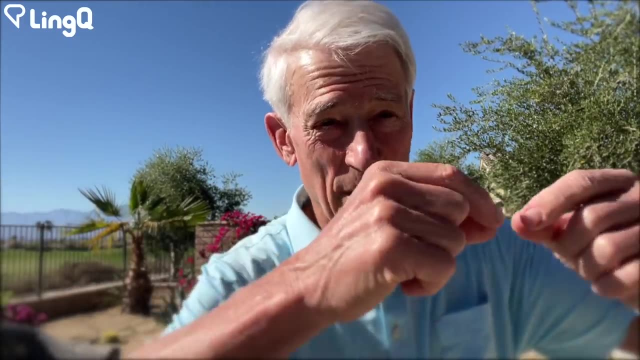 look like some fake bookshelves Or I guess another one that's fake wooden planks, but that I'll make something out of, ordered a little skinny bar so that my wife can sew a little thing and we can hang it up there, and then the lighting is all messed up and it's not working. 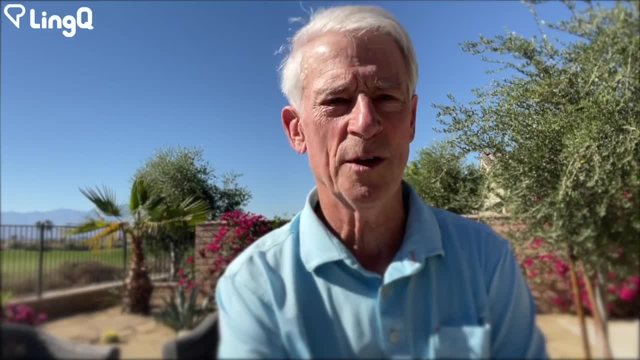 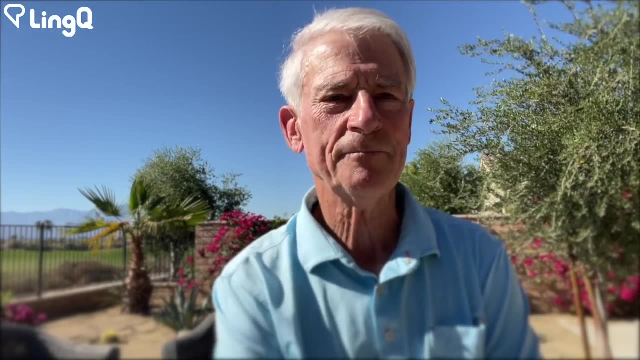 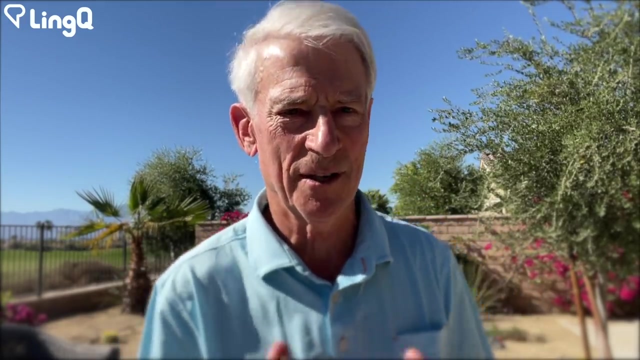 and my filmic pro is giving me problems. so I just got fed up with it, all, all my problems, and I said I'm just gonna go out in the garden and do it and I'm gonna talk about problems, language learning problems. what are the main problems that I see amongst language learners? I'm gonna try to my center. 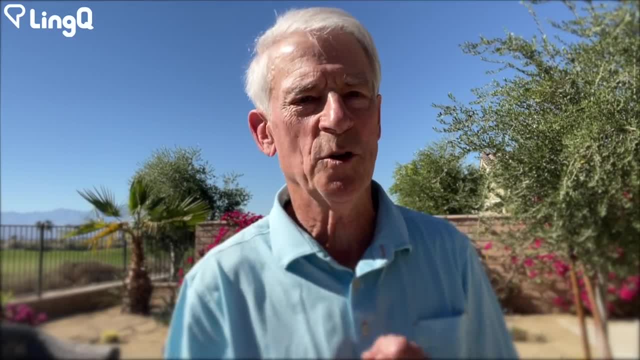 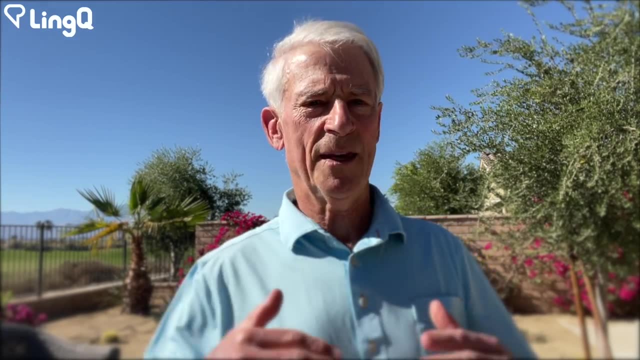 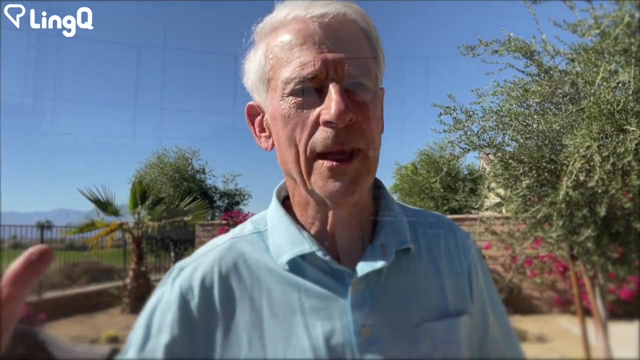 myself. here again, problems. first of all, most people don't realize how long it takes to learn a language, so people get frustrated. they get particularly frustrated when they get to that first level where all of a sudden they know a bunch of words and they realize just how little they know of the whole language. 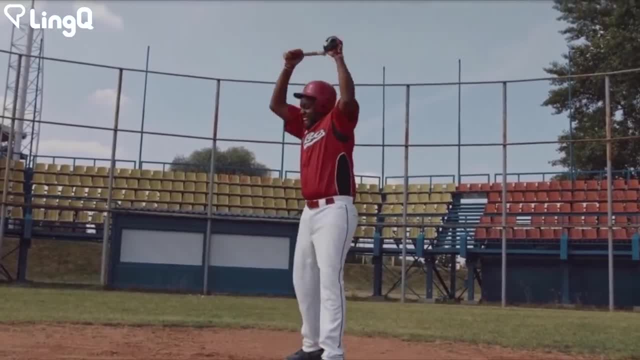 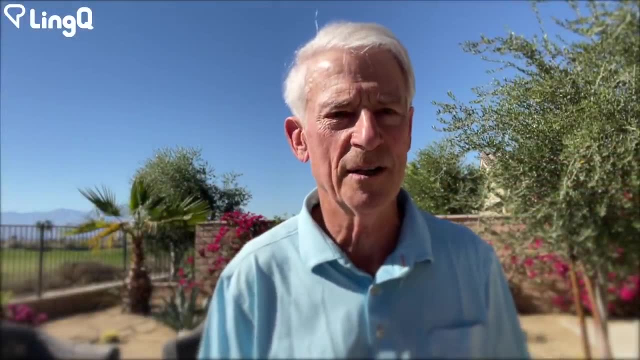 and people get frustrated and they have the sense that they're not progressing, and maybe they think that everyone else is learning and I'm not learning. and I think that's where it's so important to realize a that it's a long process and be that you have to find a way of doing it. that is. 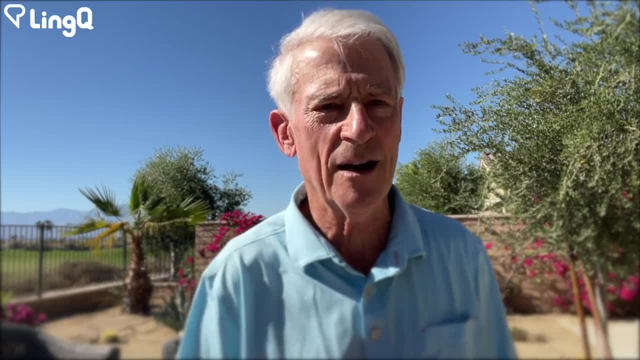 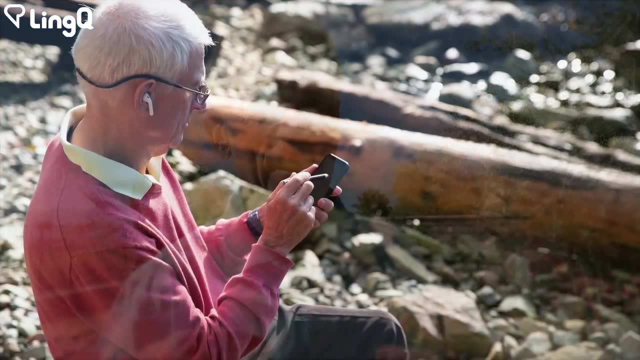 enjoyable, lungen, that you have to find a way of doing it. that is enjoyable, enjoyable. So I don't worry about the fact that I've been at Arabic and Persian for a long time and there are other people who learn faster than me. I'm enjoying it. I was listening to my 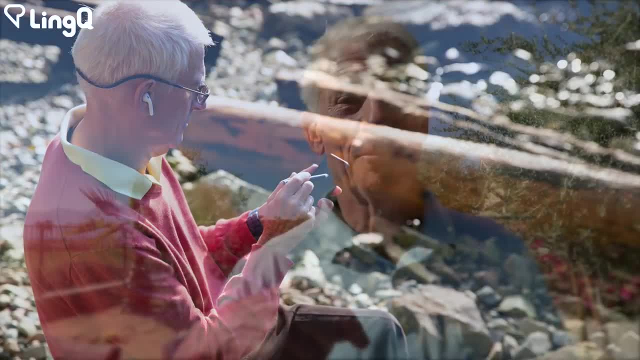 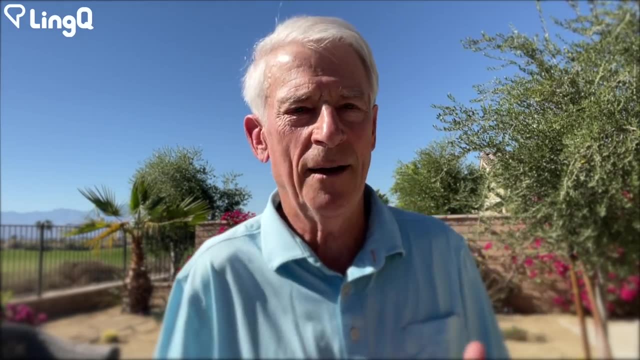 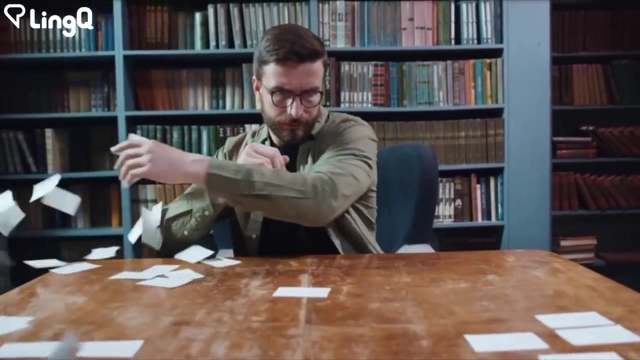 Egyptian Arabic mini stories that have been now re-recorded by Adele of Alexandria, and I was going through the texts again and it's fun, I enjoy it and I know that trickle, trickle, trickle, I'm improving. So the first thing I find is a lot of people don't have the patience. 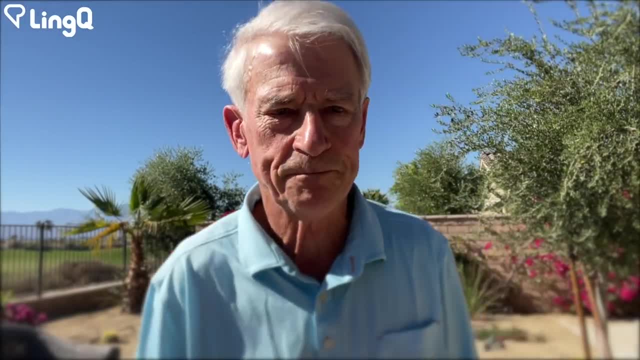 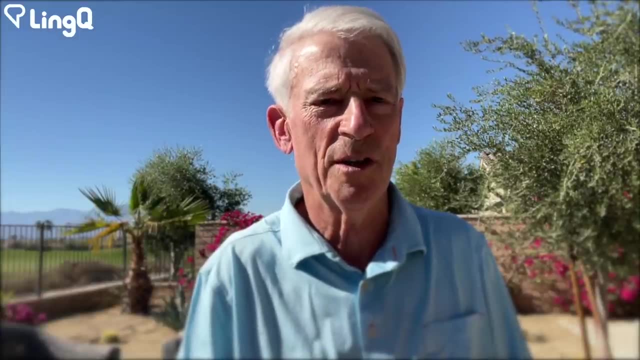 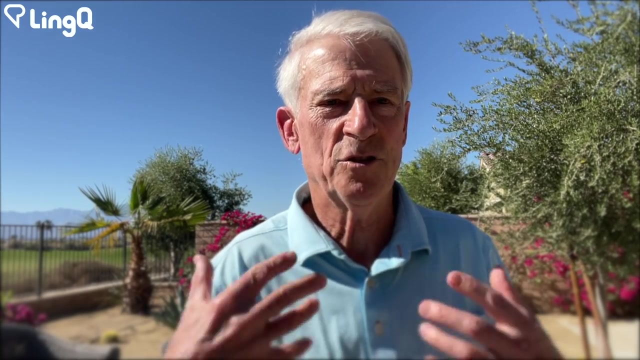 The second problem is a lot of people- and I find this myself too, you know. so I'm doing the mini stories, Adele's mini stories, and I've gone through two or three of them. It's not like instantly I've done something, like I've built something or I've made something happen, I'm just 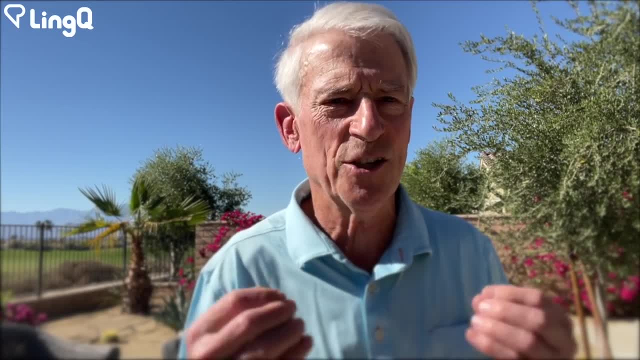 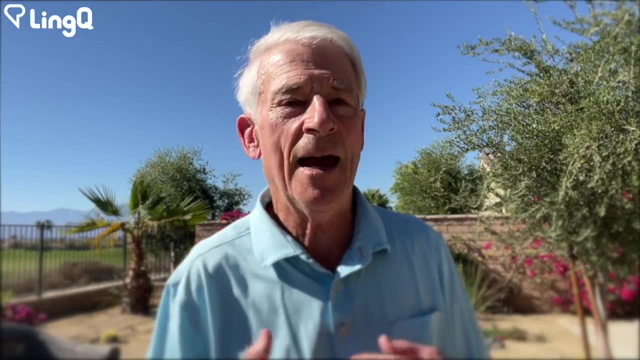 doing this and I have to remind myself that it is actually slowly. the language is trickling into me. So don't worry about doing something else. Continue doing what you're doing and do as much of it as you want. If you do 15 minutes, that's good. If you do half an hour is good. You don't have to say I have to. 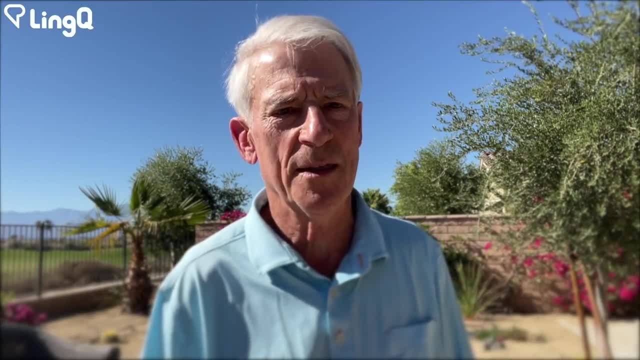 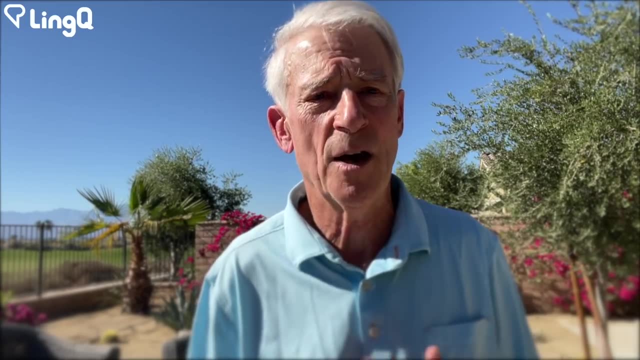 do two hours a day. Every little bit helps. So I think that's an important part of you know, making sure that the time you spent with the language, you don't begrudge yourself that time. You're happy doing it, and if it's 10 minutes, 20 minutes, half an hour, two hours, it's all good. Third problem: 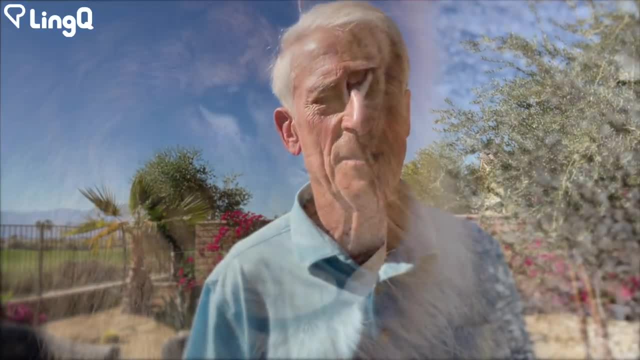 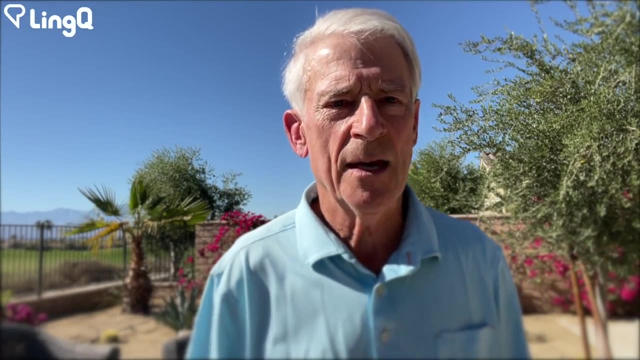 people have with language learning is they don't like to make mistakes and therefore they are intimidated, intimidated. So you know, I always stress input, but of course we all want to speak, Most people want to speak and we want to speak with as few. 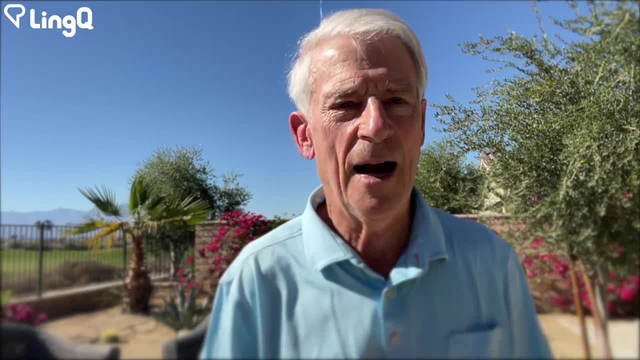 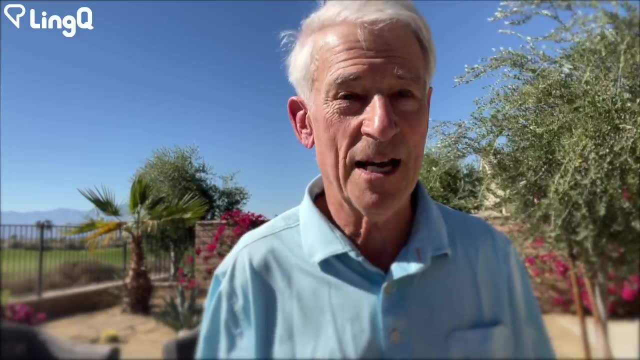 mistakes as possible. Of course. However, I like speaking with mistakes. not that I don't want to improve, but I know that if I speak with mistakes, I'm speaking, And I had a conversation this morning in German. I made so many mistakes. 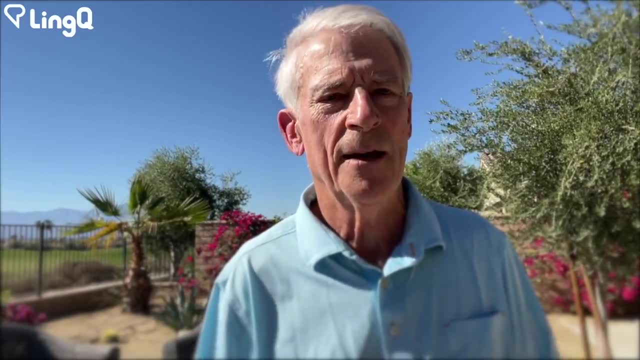 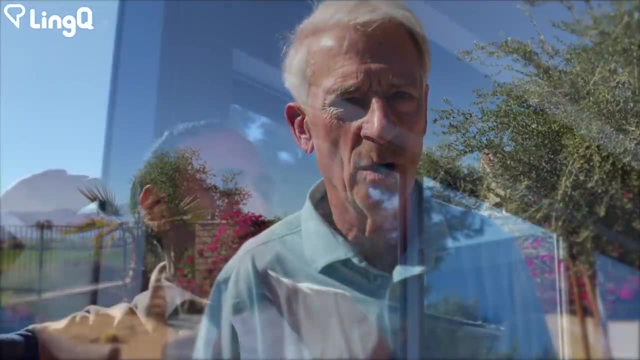 It's been so long since I spoke German and I speak it so seldom, And yet in that conversation I was getting feedback. I was getting input, we were communicating. If I were to do that more, my German would improve, not only because I'm 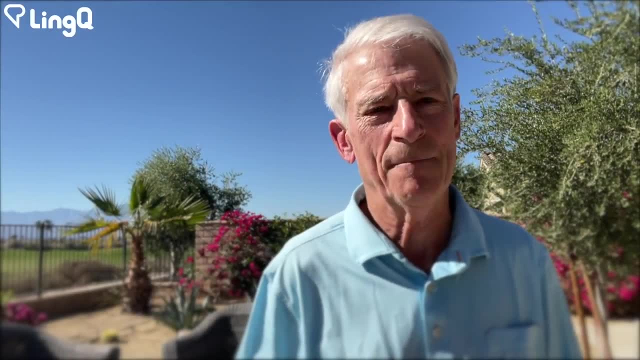 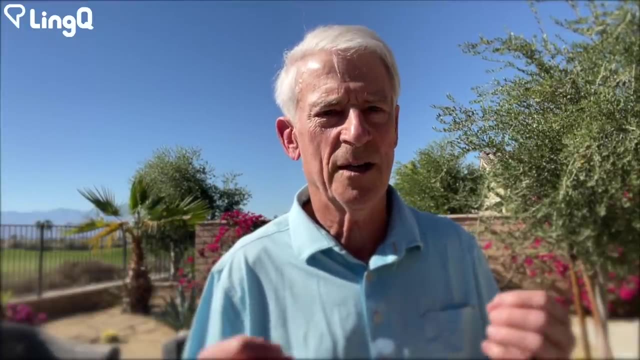 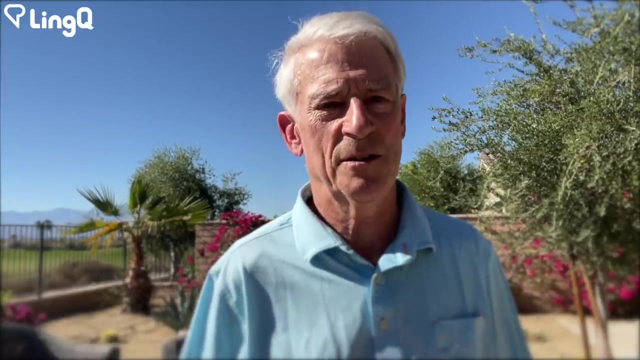 speaking, but also because I'm getting input back, and so mistakes are a good thing, mistakes are not a bad thing. Unfortunately, too often, uh, the traditional language teaching, you know instructional method- teaches us to be afraid of mistakes. Well, there's nothing wrong with mistakes. 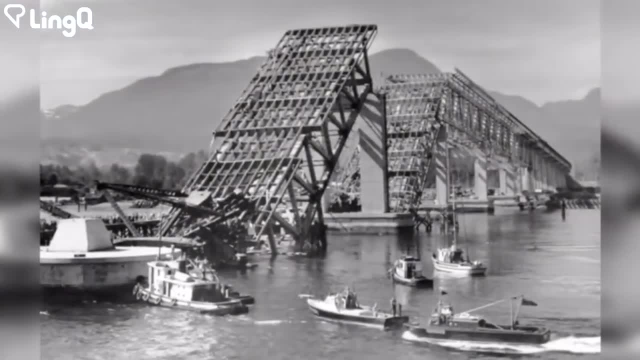 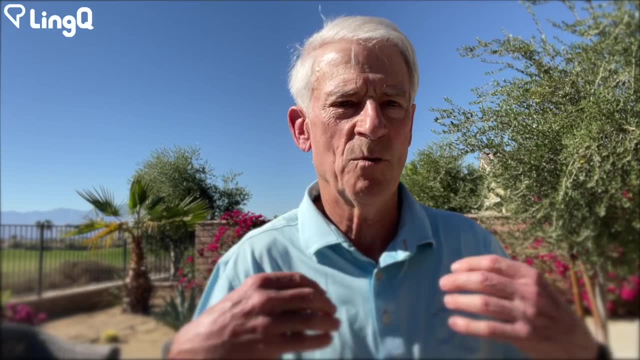 It's not like we're building a bridge, that we might design it wrong And the bridge is going to collapse. It's not like that. If we're communicating, we're already achieving the main goal, And if we want to improve, but we're not afraid to make mistakes.